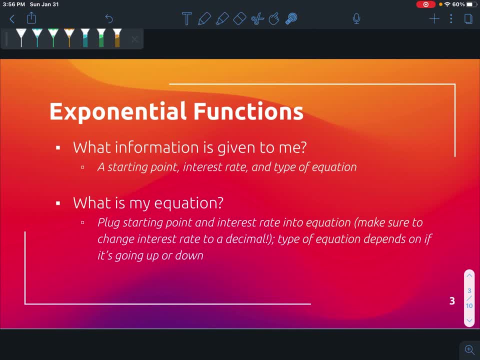 happen, though, you'll have to make sure that it is in a decimal form, so it's not always going to be given to you as a decimal, so just make sure that we are changing it to a decimal if we need to. And then, last but not least, you need to ask yourself if your answer seems reasonable. So 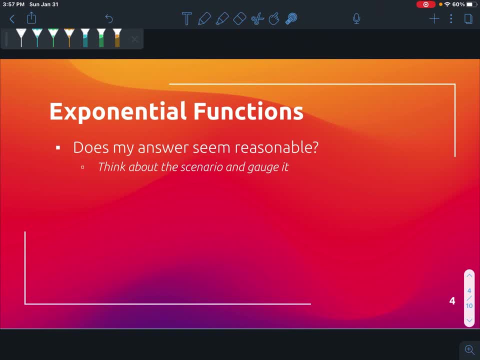 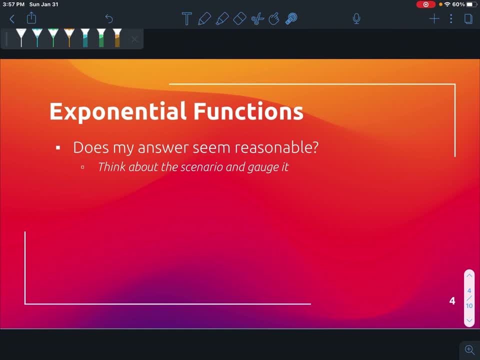 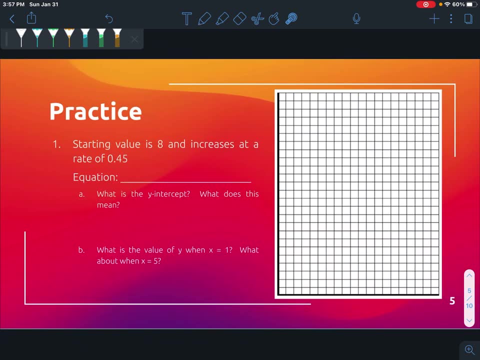 through this. So just make sure you're thinking about the scenario and that you're gauging it on your own to see if it's reasonable. All right, so we're going to look at number one here, and today we are going to graph. so in a little bit I'm going to pull up Desmos so that we can. 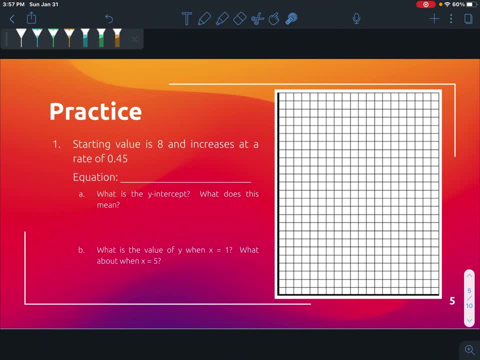 actually plug this in and graph it, but for right now let's at least write the equation. So this tells me that the starting value is 8 and that it's increasing at a rate of 0.45.. So, because it's increasing, you're going to have to use your exponential growth equation, which is: y equals c times 1 plus r to the x power. 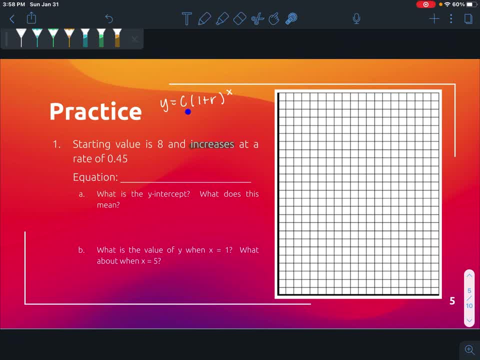 So the only things that we're going to change in this equation here are the c and the r. So my c is my starting point. That's going to be this guy right here. So that 8 is your c and then your interest rate. that's going to be the 0.45.. 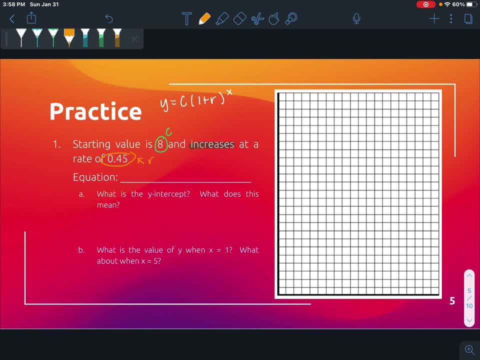 And because that one is already as a decimal, there's no percent after it, you're just going to plug that straight in. So then our equation is going to look something like: y equals 8 times 1 plus r, which is 0.45 to the x power. 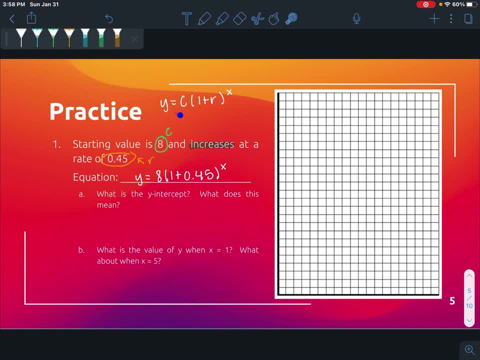 So again, notice the only thing. So the only things I've changed. I've changed that c to be the 8, because that's my starting value, and I changed the r to be this 0.45, because that's the rate. 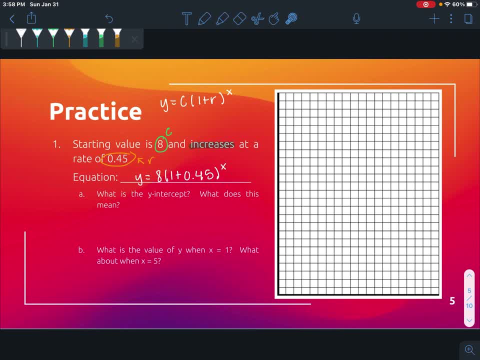 It tells me that that's the rate, And again it's increasing. so that tells me I need to use the equation with a plus in it. So now let's go ahead and graph this. I am going to pull up Desmos here and we are going to plug in the equation and graph it. 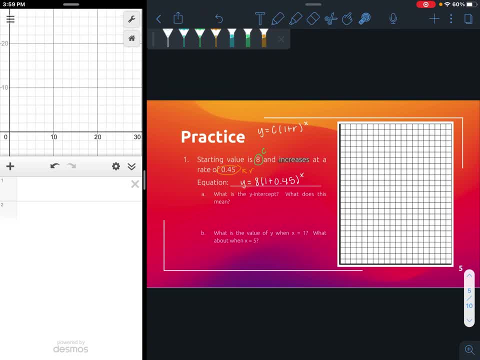 So if you have anything already in there, any equation that you've previously graphed, get ready, Get rid of that, And now to plug it in, just type it as you see it, So it's going to be y equals, and then parentheses, 1 plus 0.45.. 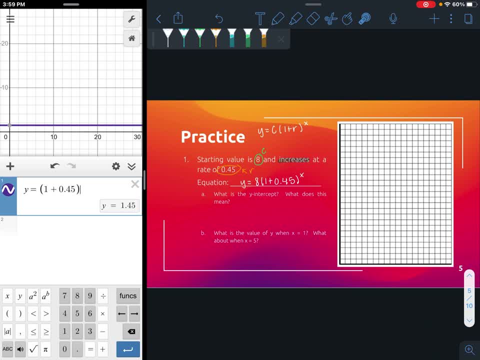 And then close your parentheses. Now, to get that x, you're going to click this a to the b button that I'm highlighting right here. So it's a to the b and that will give you an exponent, and in there you're going to put x. 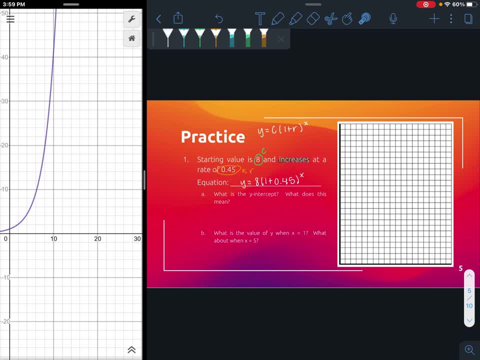 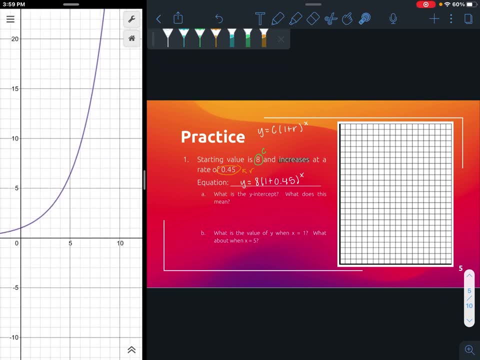 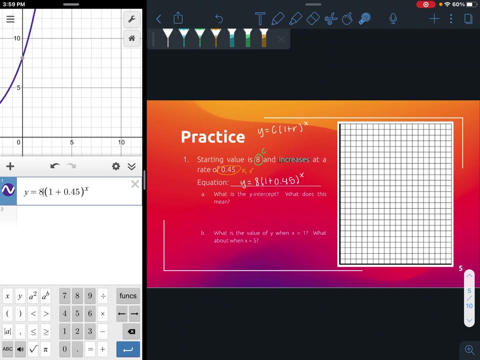 So then this will be the equation, So this is the equation that we're going to use for this problem. Now, this is a pretty steep equation, And actually, if I'm looking at this, I think I've missed my 8.. I apologize for that. 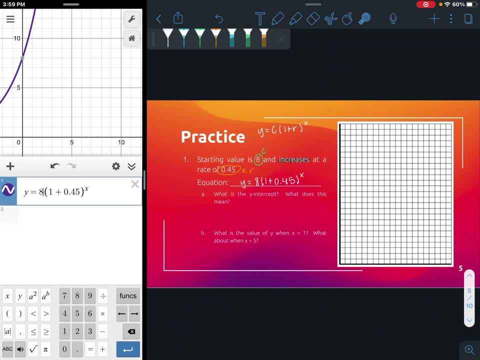 There should be an 8 out front, So this should be your equation. My apologies, So it should look like this now, which looks a little bit better, But it's still a pretty steep equation if you zoom out and look at it. 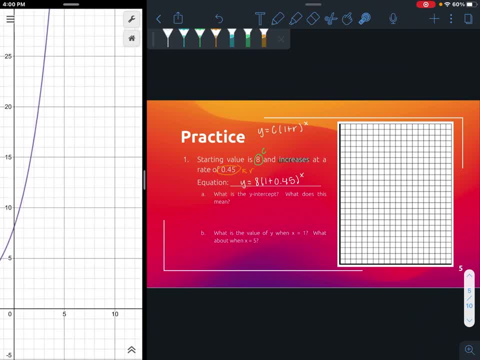 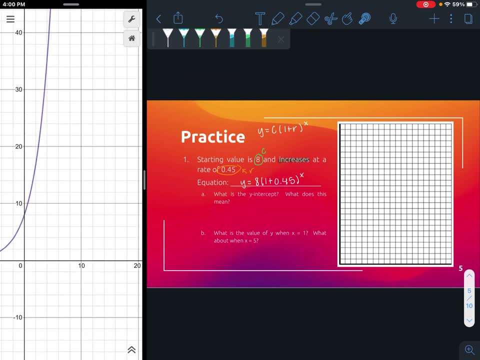 We're just going to do a very quick little graph. Your graph is going to go all the way up to 25.. But you'll notice that your graph goes way, way farther than 25.. That's what it means to grow exponentially. 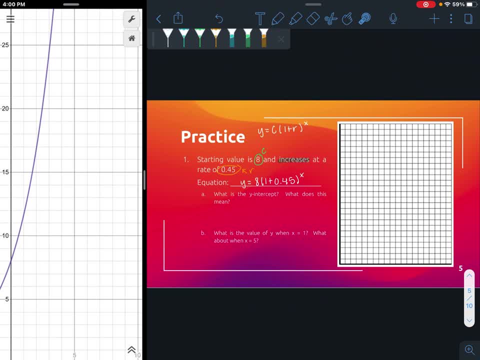 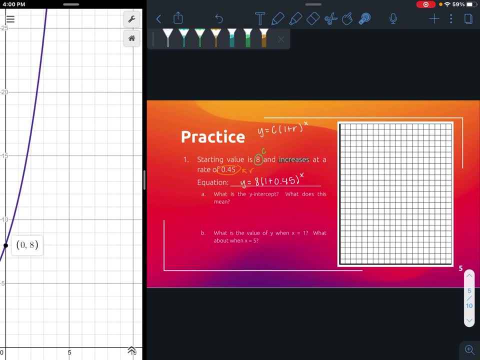 So I'm just going to basically pull it up so that it's kind of like this, And this is the window of the graph that I'm going to be looking at here. So this y-intercept, if you click on that, that's 0, 8.. 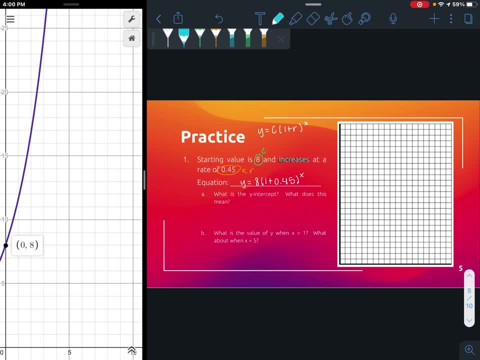 So when you plug that in or you put that over on your graph here, 2, 3, 4,, 5, 6. 7, 8.. I'm just going to count 8 up And I'm going to put my dot right there. 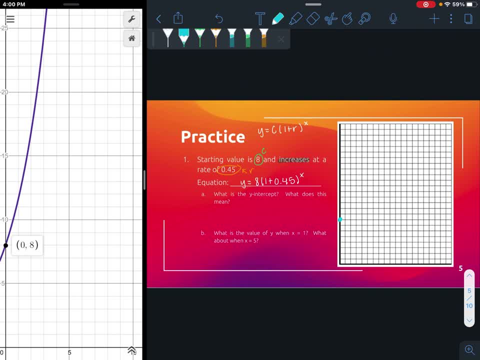 And then you're just going to draw a line as best you can. It doesn't have to be super, super pretty, But it would look something kind of like that. So then we want to know what the y-intercept is, And we've already said that this one here is actually 8.. 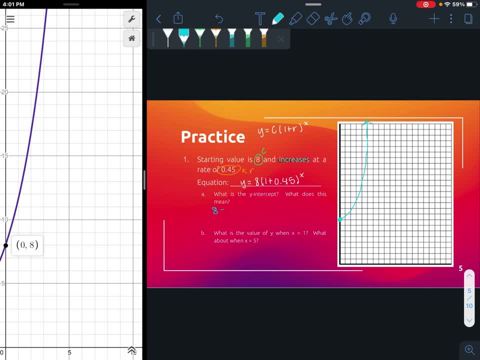 We found that from the graph, So it's 8.. And what does that mean? Well, that just means it's the starting point. But we already knew that. I just wanted you to see what it looks like, What it looks like on the graph. 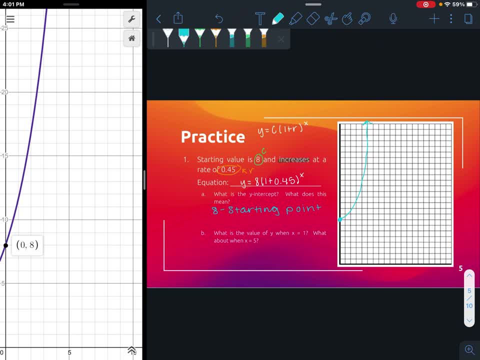 And then we want the value of y when x equals 1.. So, just like what we did with the quadratics, you're just going to trace the function And you'll see all of these values. So I'm looking for when the first number is 1 or very, very close to 1.. 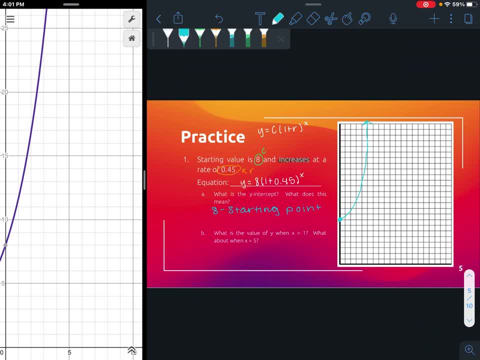 And I think I just about got it right here, And that's at 11.6.. So when x equals 1,. y equals 11.6, which is still on my graph Now, if we want to look for when x equals 5,. 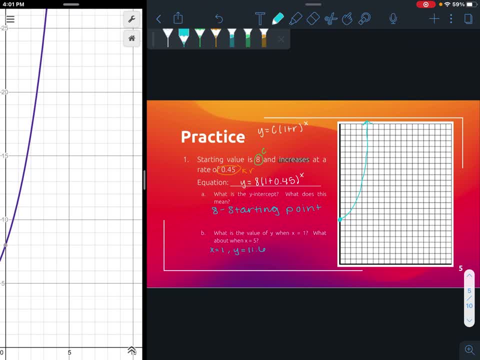 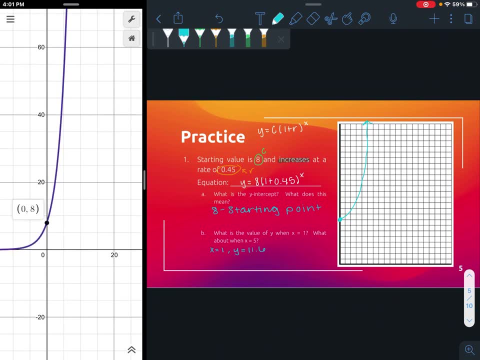 I can keep going up here, But if you'll notice, it's actually really far off my graph, So you're going to have to zoom out quite a bit to get there, And that's okay. So just click on the graph again. 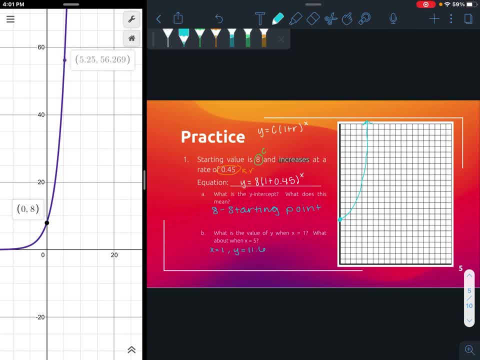 And then just go on up until you reach 5.. So 5 is right about in here. It's at 51.278.. So when x equals 1, y equals 11.6.. So that's at 51.278.. 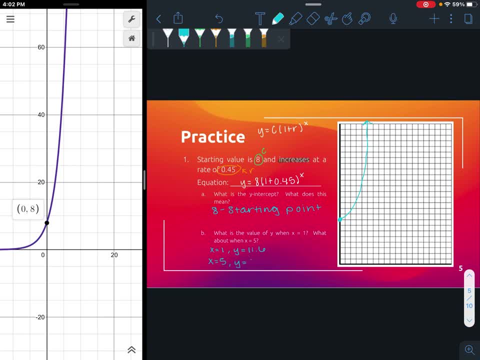 So when x equals 1, y equals 11.6.. So that's at 51.278.. So that's at 51.278.. 5y is 51.278 or something like that. So just something to look for as you're doing those. 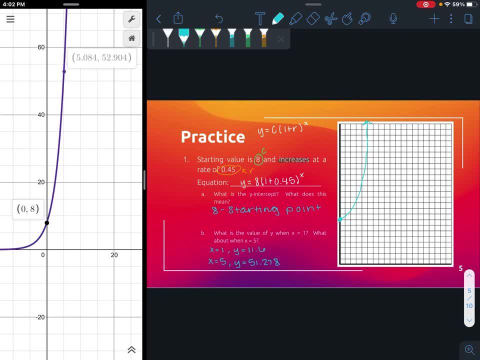 I will say that sometimes it's more inconvenient to look at the graph than it is to just use the equation, which is why we're going to look at both ways today. We're going to just do a couple with the equation, I'm sorry, with the graph. 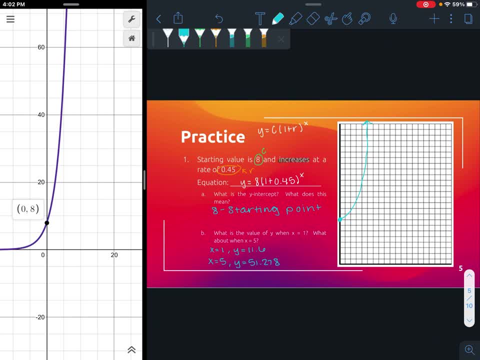 But then we're going to really focus on learning the equation and how to solve it, and how to solve it with that Oops. So let's look at number 2 here: Same exact thing, just a different problem. So we're told that the starting value is 23,. 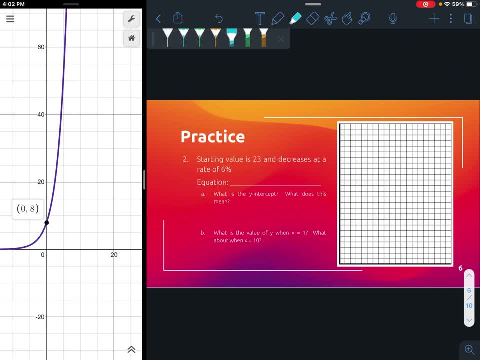 and it decreases at a rate of 6%. So I notice it says decreases, which means I'm going to use the equation that has the minus in it. So that would be: y equals c times 1 minus r to the x. Now your c is going to be your starting value. 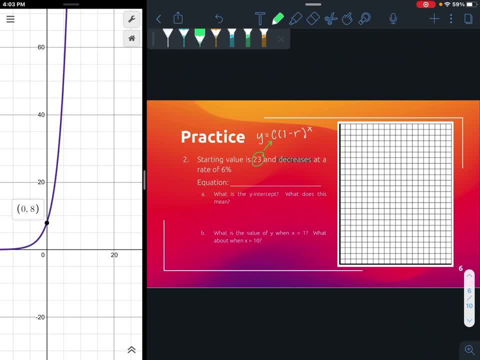 so that's the 23.. That'll get plugged in right there. And then the r. this time I'm told that my r is 6%, So over here I'm going to write that out: 6%. If you're given a percent, you have to change that to a decimal. 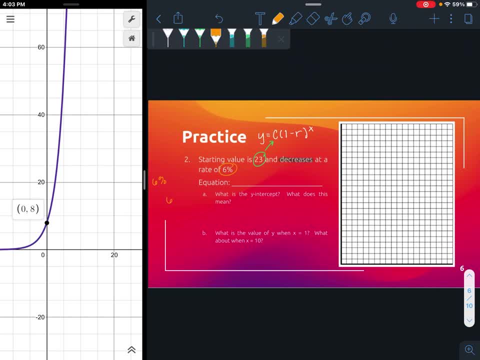 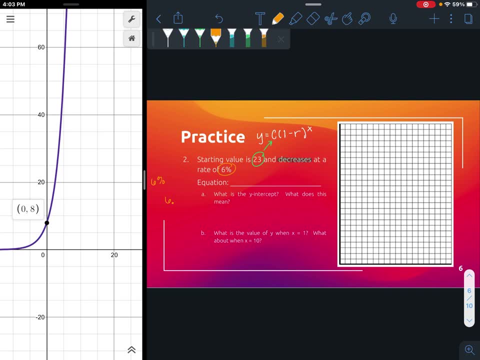 To change that to a decimal. you're going to take your 6, or your percent or whatever, and the decimal point is currently after the 6.. If it's a whole number, it's just right there. after that number You need to move that decimal place two spots over. 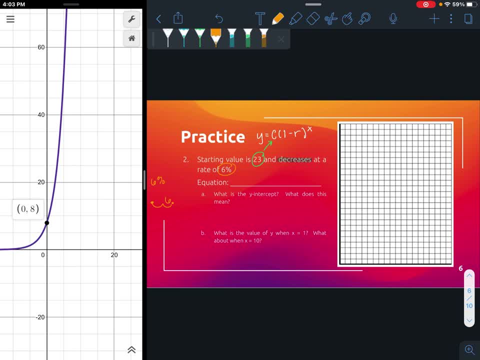 and now it's going to be over here. So to fill in that slot, you're going to actually put a 0. So this r is now 0.06.. So that's what's going to get plugged in to your r up in here. 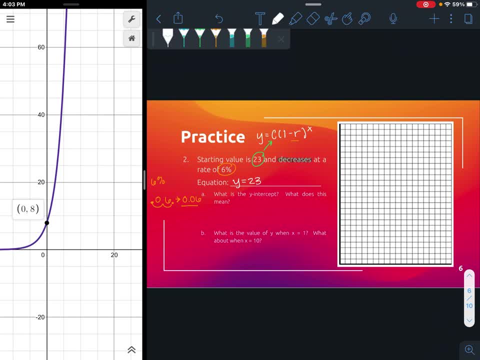 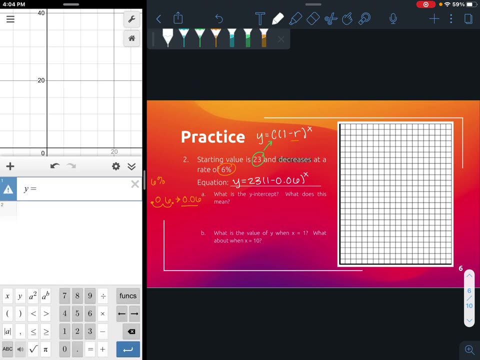 So my equation then is: y equals 23 times 1 minus 0.06 to the x power. So that's what I'm going to type in over here on my graph. Get rid of that equation here. So y equals 23 parentheses, 1 minus 0.06 parentheses. 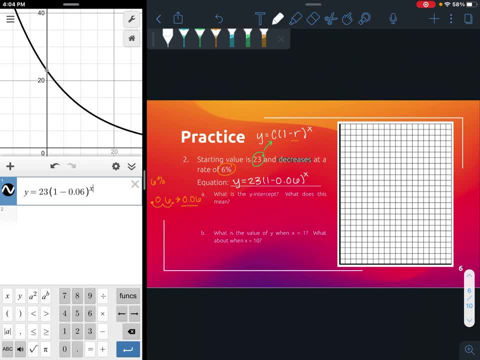 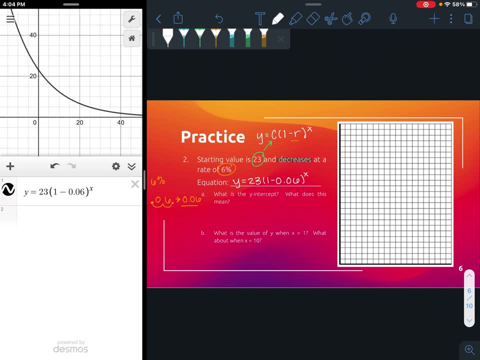 And then you click that A to the B button and then you can put your x in there and then that's your equation. So if you'll notice that this equation is not quite as steep as the other one was, The other one shot up a lot quicker. 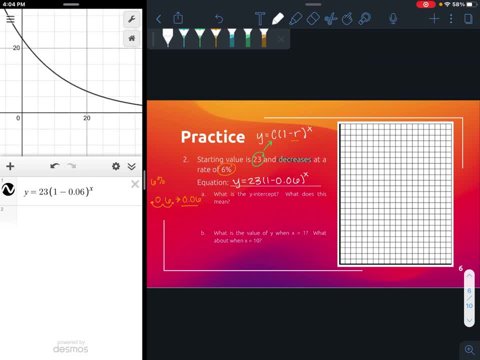 This one here is a lot nicer. It comes down. It's at that nicer angle or at that nicer degree there. So I'm going to graph this real quick. 23 is your starting point, right? I mean, if you click on your graph over here, you can get to that 0.23.. 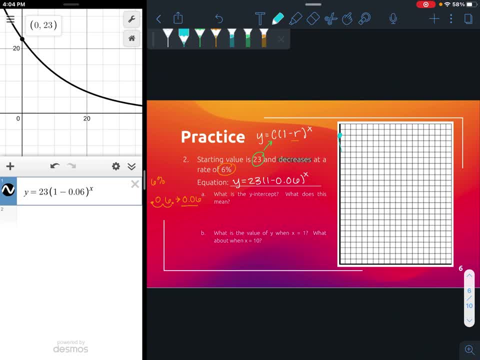 That's your starting point, And then I just want you to draw a nice gradual curve off there. Again, it doesn't have to be perfect, I just want to see a general picture of the graph itself. So what is the y-intercept? 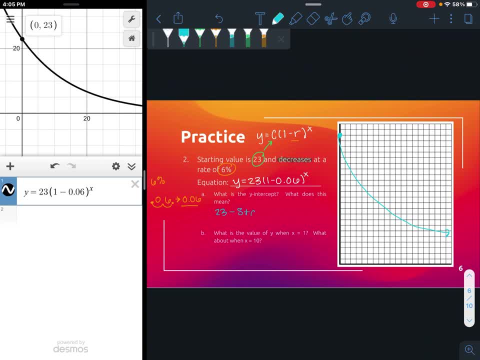 Again, we know that this is 23,. and this is the starting point, Just Just like we talked about last time. So that's your starting point, or your starting value. Then I want to know what the value of y is when x equals 1,. 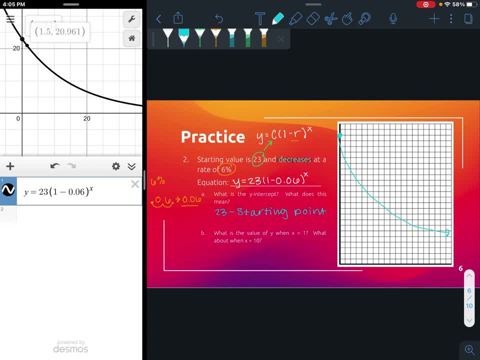 and when x equals 10.. So when x equals 1, it looks like it's about. It's about 21 point, something it looks like, Maybe like 21.62, it looks like So when x is 1.. 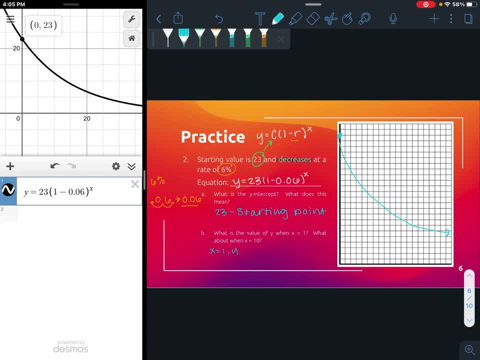 When x is 1, y equals 21.62.. And then when x equals 10, let's move our cursor down here. It is about- It looks like 12 point something. I think that's about 12.38 or something like that is what I figured out. 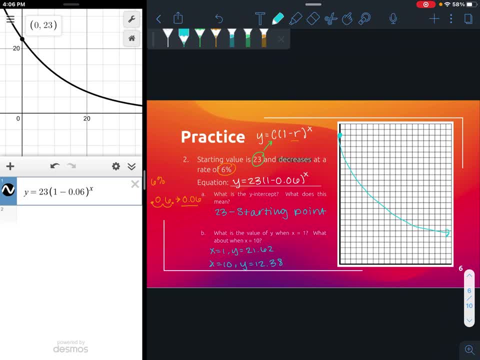 So 12.38.. So, if you'll notice, this one here decreases at a much, Much Slower rate, which makes sense, because in our last equation the rate was 0.45.. And in this one the rate is 0.06.. 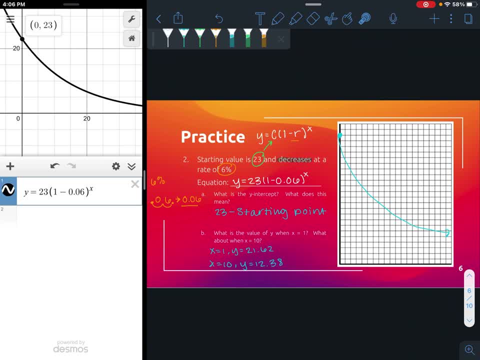 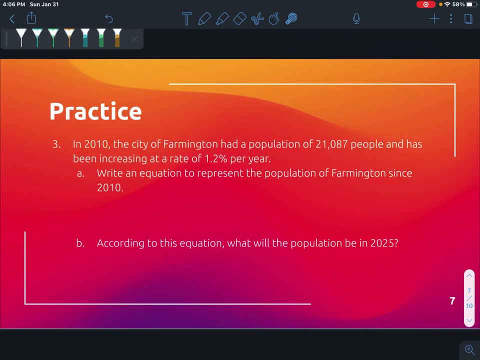 So it is a more pronounced difference there. Let's take a look at some problems without graphing. So in number 3 here we have a word problem. It says: In 2010, the city of Farmington had a population of 21,087 people. 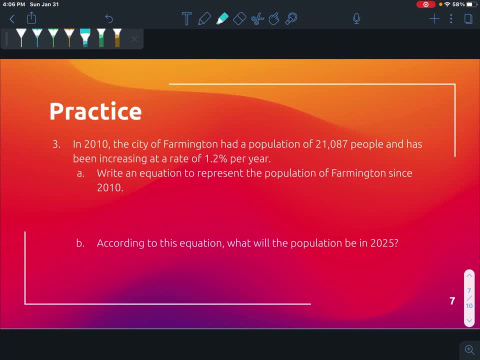 and has been increasing at a rate of 1.2% per year. So I see increasing right, Which means I'm going to have to use my: y equals c, and then 1 plus r to the x. So I need to write this equation. 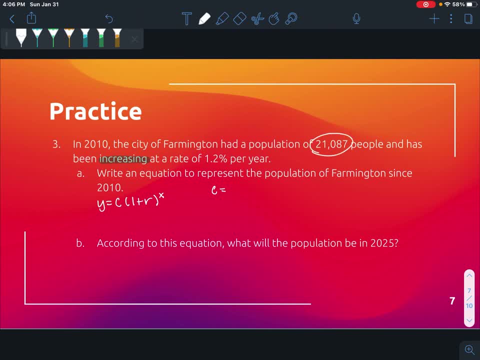 So c remember that's your starting point, which is going to be this guy right in here. It started at that part at in 2000. at least That was what the population was. So 21,087 is my c. 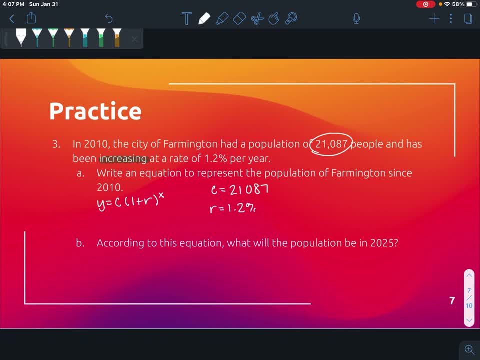 And then my r is my 1.2%. Now, be careful with that. Again, we need to move the decimal place over, So it's going to be 1.2, but then you need to move this over one, two spaces. 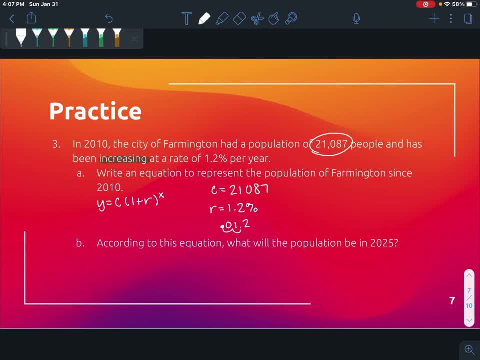 So your new decimal point is going to be over here, and then put a zero in as a placeholder, So now your r is 0.012.. So then the equation that I'm going to write should look something like: y equals 21,087. 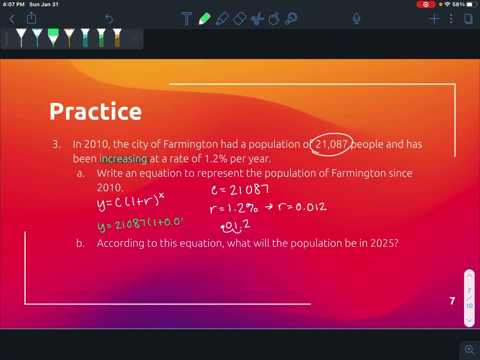 Times 1 plus 0.012.. And then we're going to keep that to the x power. So this is the equation. This is your answer for part A here. Now part B. I'm going to use that equation and I want to predict the population in 2025. 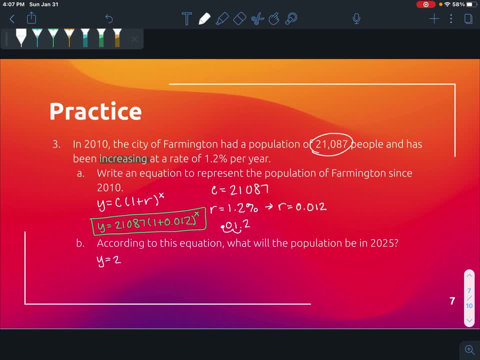 So I'm going to rewrite my equation down here. So it's 21,087 times 1 plus 0.012.. To the x. So to predict this, now you can type this into a graph, But I will tell you that graphing with such big numbers, 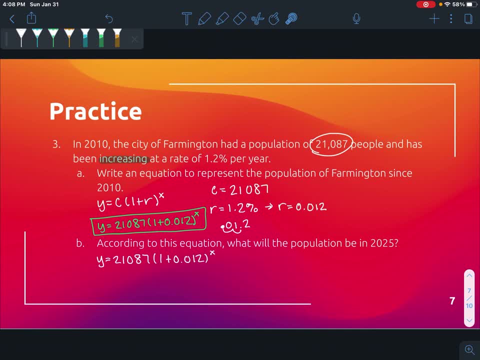 is a lot more complicated. So we're just going to do the really easy thing and plug it into a calculator. To do that, we need to figure out what to put in for this x. Okay, and this x is going to be your time. 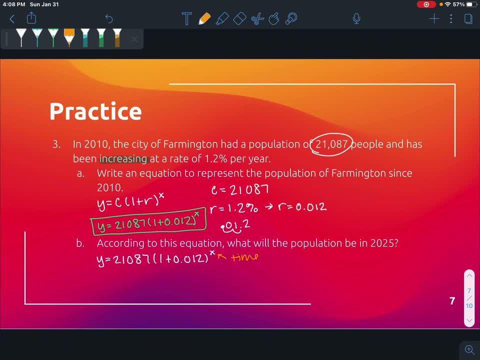 So I'm going to make a note of that real quick. That's your time that is passed Now. a lot of people are just going to want to put in this, but be careful. This would say that you're looking for the population after 2025 years. 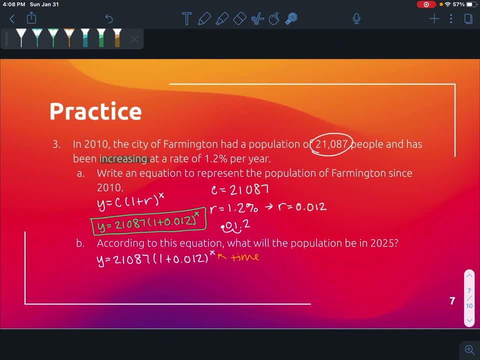 but we're just looking for the time since 2010.. So you're going to take the year that you're looking for, which is 2025, and we're going to subtract the initial starting year, which is 2010,, and that's going to give me 15.. 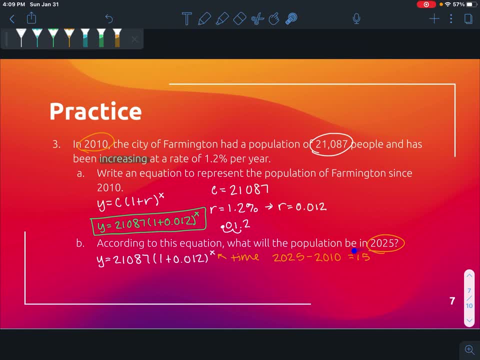 So we're looking for how the population has increased over the past year. So we're going to take the year that you're looking for and we're going to subtract the initial starting year within the last 15 years or so. So when I type this into a calculator, 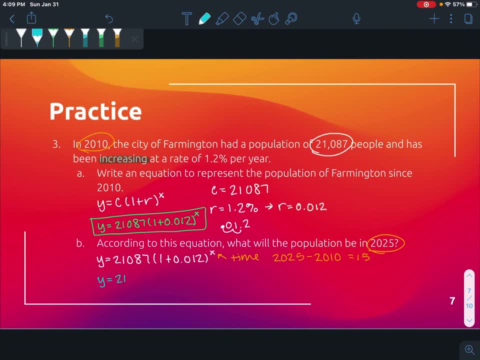 I'm going to write it down here. You're going to type this in just like you normally would- keep the parentheses and everything like that- but to get that exponent you're going to use this upward arrow key or upward caret key, we sometimes call it. 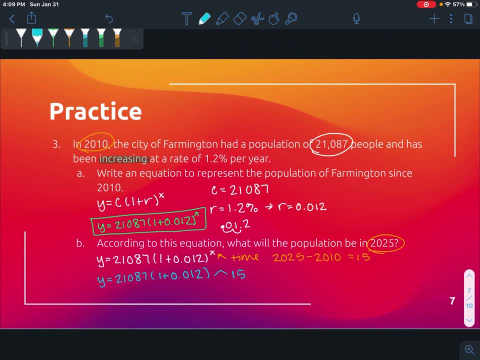 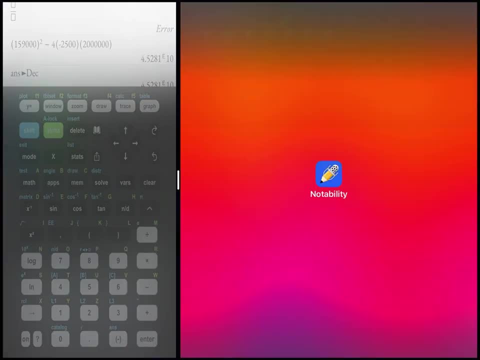 and then you're going to put the 15 in there. Now, if you don't have a calculator like a scientific calculator, the one that I recommend is called TACI, and I'm actually going to pull it up here so that it's on the side of my screen. 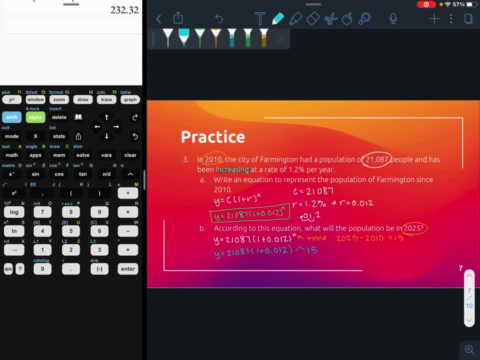 So it'll look something like this, and I'm just going to type this in right here, exactly as I see it, and we'll get our answer. So: 21,087, parentheses 1 plus .012,. close off the parentheses. 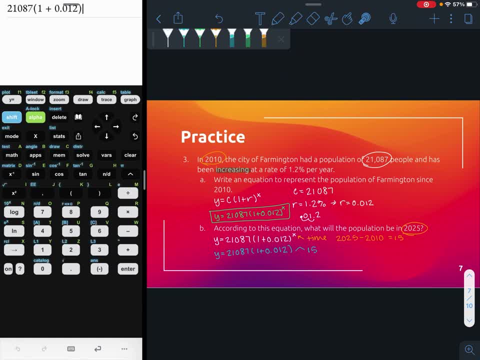 and then the upward arrow key is right above the division symbol. It's right up in here, Oops. and so that's going to give me oops. there we go. That's going to bring up that exponent piece, and then you'll plug in a 15.. 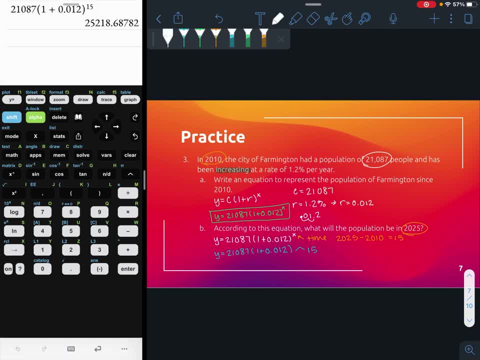 When you click enter, that will give you your response. So my answer, then, is 25,218 people. We're not going to round up for this one because we haven't gotten to the 2,000, or, I'm sorry, the 25,219 people. 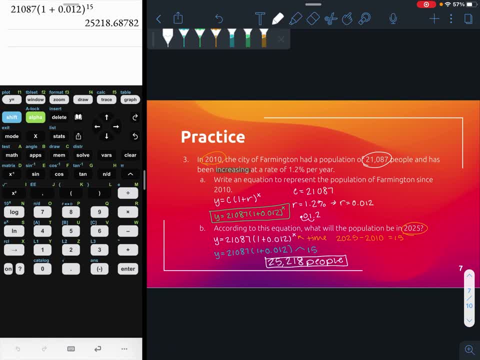 That would happen later, but you can't have 0.6 of a percent or something like that, so we're just going to keep it as this, right here. If you have any questions about this stuff, let me know. We are here to help you. 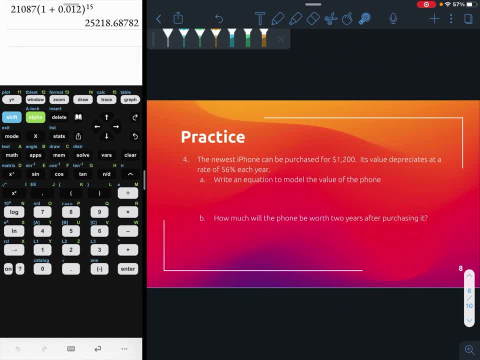 Let's do one more word problem before we send you off to do your homework. So number four says that the newest iPhone can be purchased for $1,200.. Its value depreciates at a rate of 56% each year. This word depreciates means that you're going down. 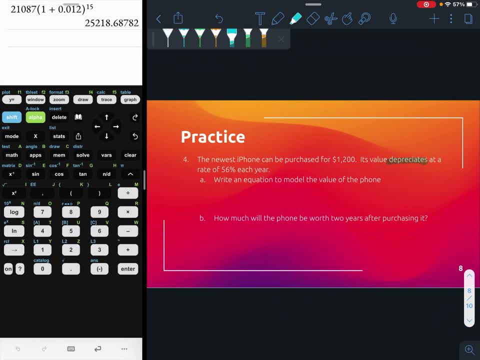 It means it's declining. Uppreciate is the opposite of that. So uppreciate would mean to go up, Depreciate means to go down. Because it's depreciating, I'm going to use my exponential decay function And I'm just going to start over with that. 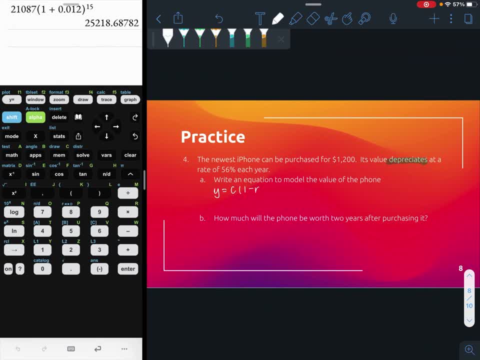 So it's: y equals c times 1 minus r to the x power. I need to figure out what my c is and what my r is. My c is this right here. That's what you're going to plug in for c, And then your r is this: 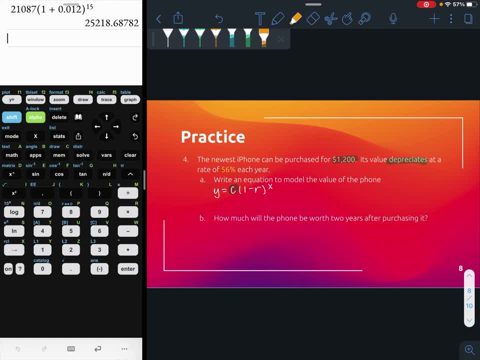 But you have to do a little bit of work before you can plug it in for r. So my c again that's 1,200.. And your r is 56%. But you have to move that decimal place over two spaces. 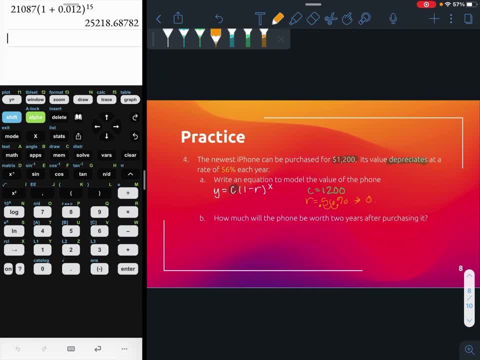 It's going to be right in front of the 5.. So your rate is 0.5.. That's what you're going to plug in for c, And then your r is this: That's what's going to get plugged in right here for this r.